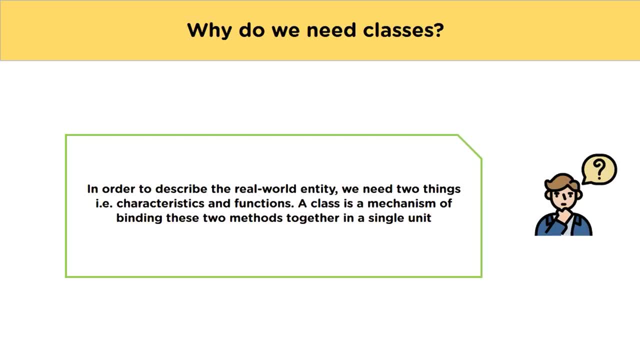 and destructors. So, first is, why do we need classes? To understand this, we need to know that C++ is an object-oriented language And it also introduces the concept of real word entities. So in order to describe the real word entities, we need two things, that is: 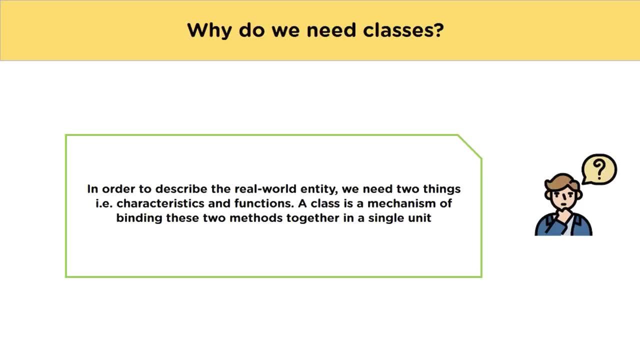 characteristics and functions, And a class is a mechanism of binding these two methods together in a single unit. Also, class has its own members, like functions, variables, constructors, destructors, etc. which are commonly used in C++. And class has an important 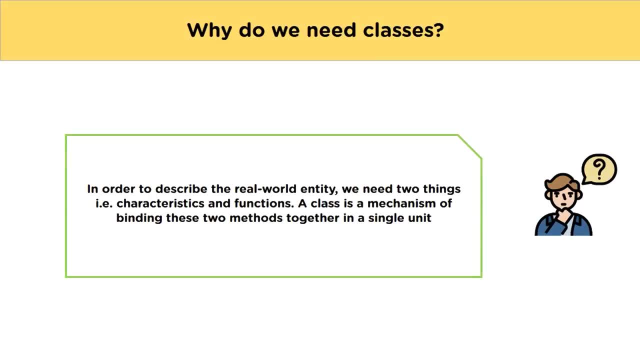 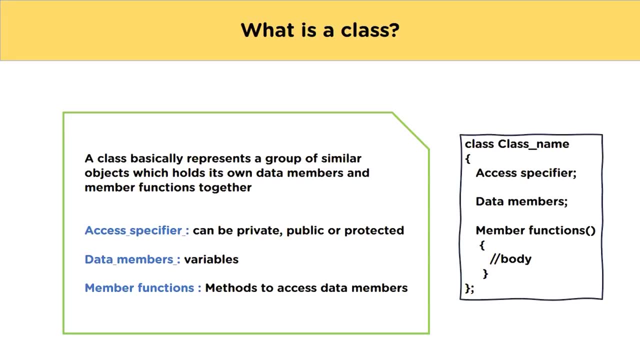 role in the concept of inheritance as well. Now let's understand what is a class. Classes are one of the most important features of C++. that leads to object-oriented programming. It represents the set of properties that are common among all the objects of same type. 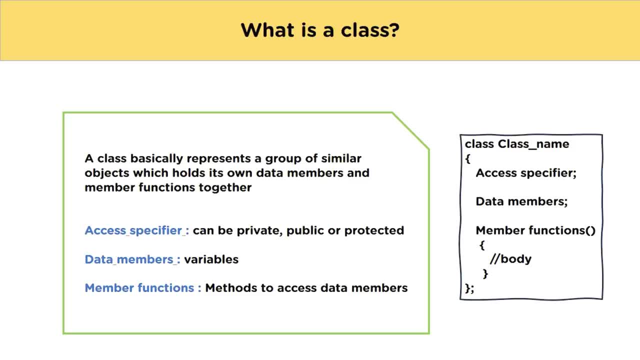 A class basically represents a group of similar objects which holds its own data. members and member function together, And this is the basic syntax of a class. First is class keyword which is used to create class. Then after that we will write the name of the class. 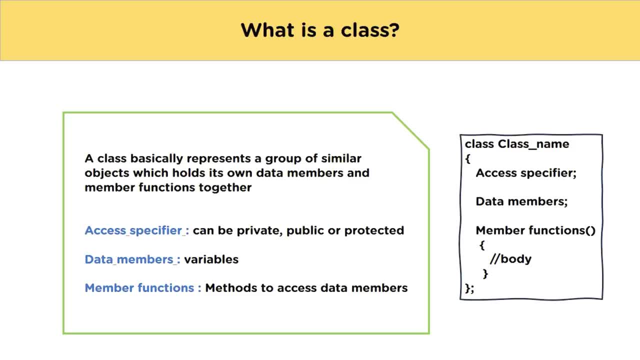 Then inside the name of the class, there is access. passivar- that can be private, public or protected. After that there is data members, that is, objects of the same type. After that we will write the name of the class. Then inside the name of the class, there is access. 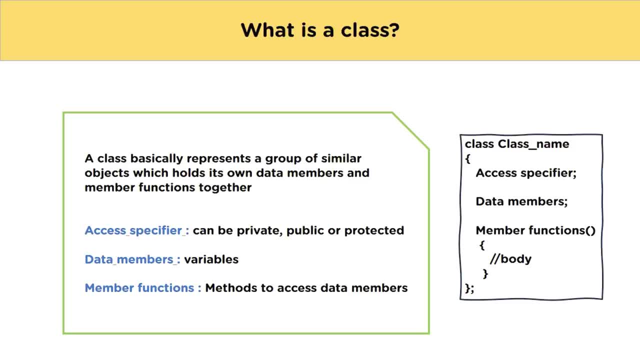 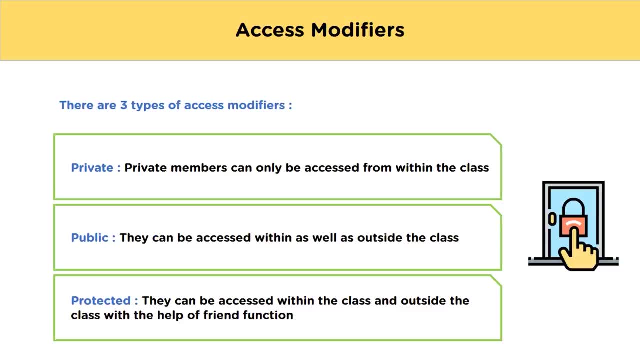 variables, that is, the variables And then the member functions And also class body- must be surrounded with braces. Now let's discuss access modifiers. It basically grant permission or set the restriction for data members of the class. Access modifiers in a class are used to provide accessibility to the class member, For example in a school. 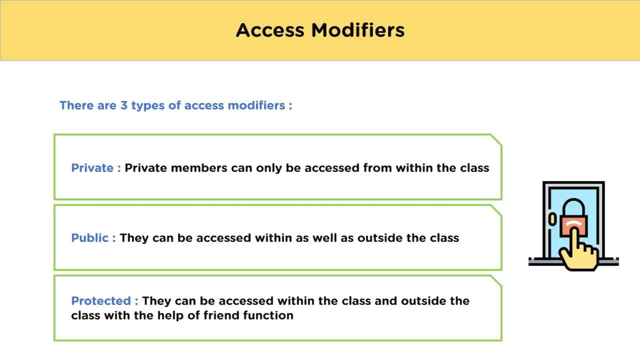 teachers are allowed to see the question papers before the exams, but the students are not allowed to do so. anyone other than teachers cannot access those questions. now we can relate these teachers to data. members of class which have access and students are outside functions that do not. 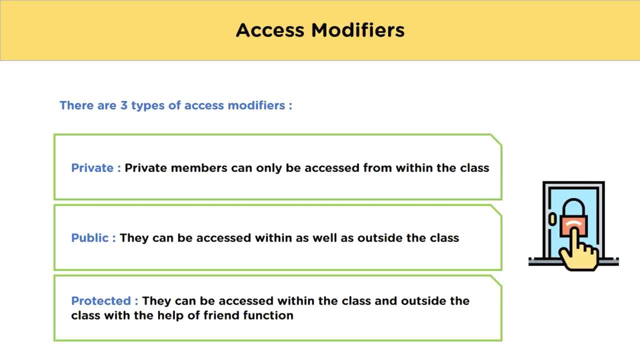 have the access. so there are three types of access modifiers: private, public and protected. private members can only be accessed from within the class. that means outside data members and member functions cannot access it. public, as the name suggests, it can be accessed from within the class and from outside the class as well. protected members can be accessed from within the class, but. 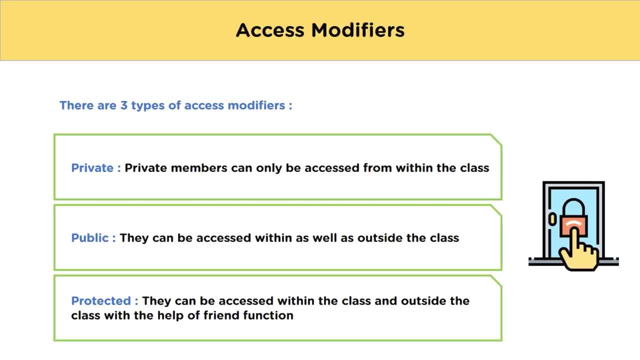 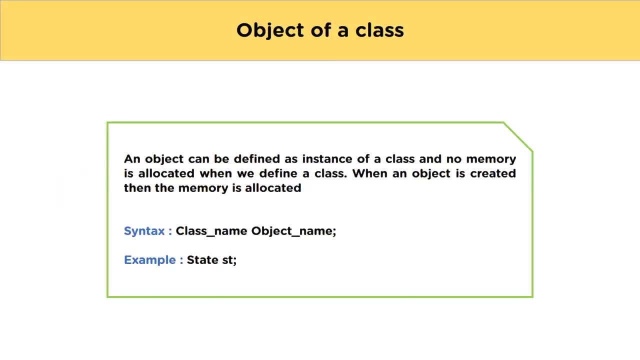 cannot be accessed from outside the class, but with the help of friend function, it can be accessed from outside the class as well. now let's learn about object of a class. an object is an instance of a class. it is a real word entity that contains state and behavior of the class. 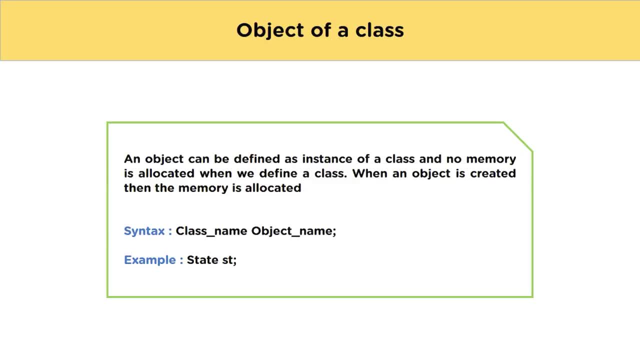 when we create an object of a class, then the memory is allocated, and no memory allocation occurs when class is defined and we can create as many objects of a class as we need. in this example, state is the class and st is the object name or reference variable. so this is how. 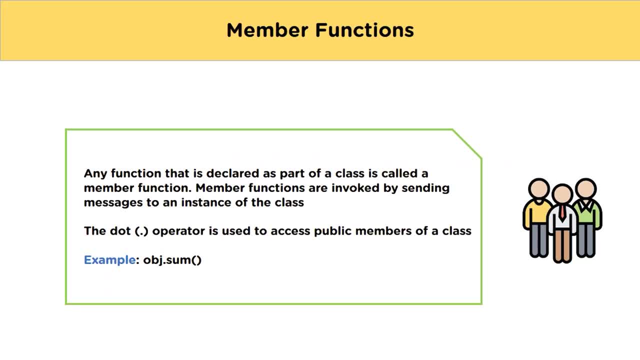 an object is created. now coming to member functions. member functions are also known as methods. these are as much as possible as part of the class as the member variables. these member functions can be invoked by sending messages through an instance of a class, with the help of dot operator. for example, if the name of 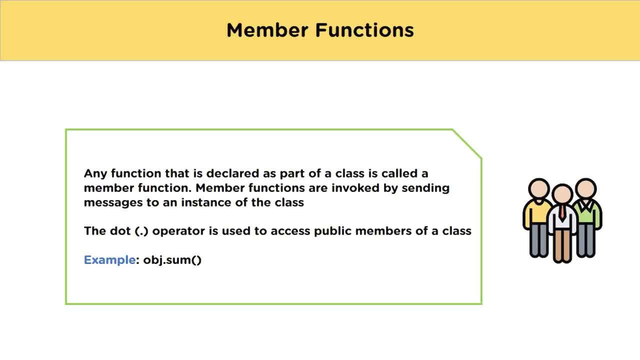 the object is obj and we want to access a function named sum, then it will be obj dot sum. here, obj is the name of the object and sum is the name of the function. now let's learn about constructors. constructors can be defined as a special type of method. 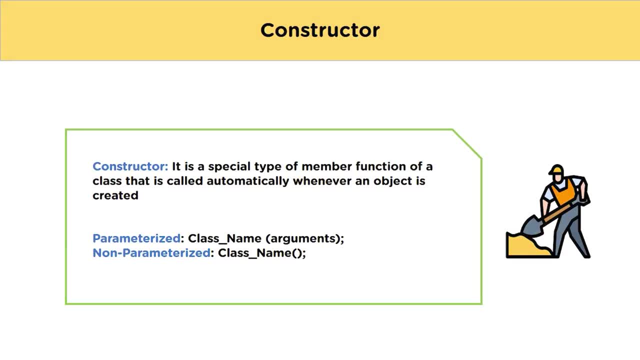 that is invoked automatically whenever an object is created. its main use is to initialize objects. it doesn't have any return type and a constructor has the same name as that of the class and it is of two types: parameterized and non-parameterized. the syntax for parameterized constructor is class name, which is a constructor name, and then 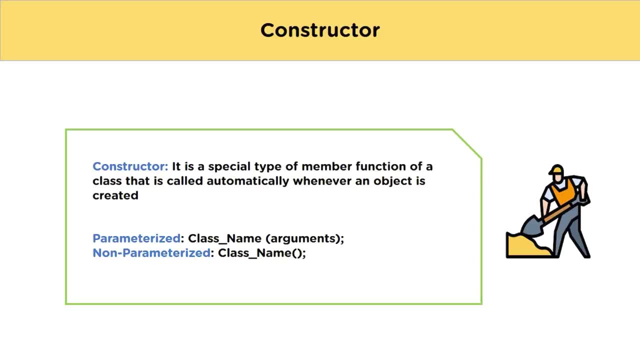 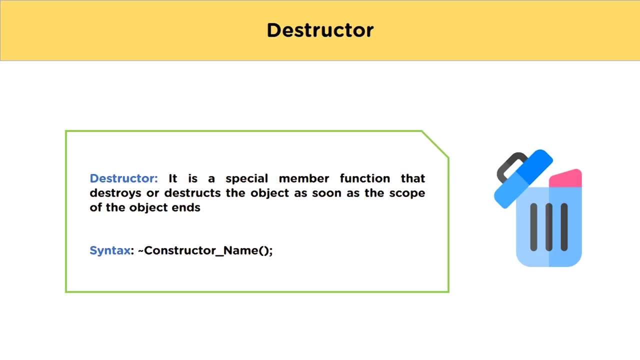 arguments inside the bracket. in non-parameterized constructor, the syntax is class name with empty brackets as there are no parameters in non-parameterized constructors. now, after constructor, let's discuss the destructor also. destructor, as the name suggests, is also a special method that destroys or destructs the object as soon as the scope of 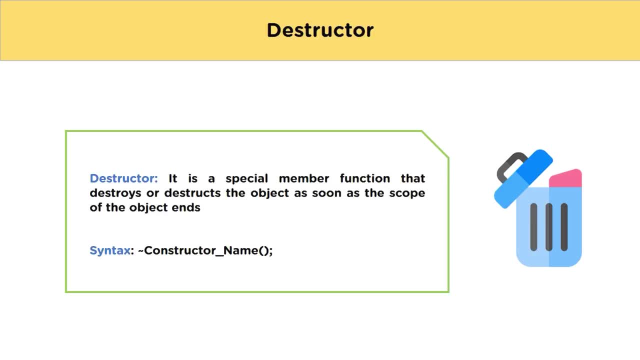 the object ends and it is automatically invoked when the object goes out of the scope. its name is same as that of the class, but with the tilde sign. here is the syntax of destructor tilde sign with constructor name or class name and then empty brackets. now to do some examples on classes, let's move on to. 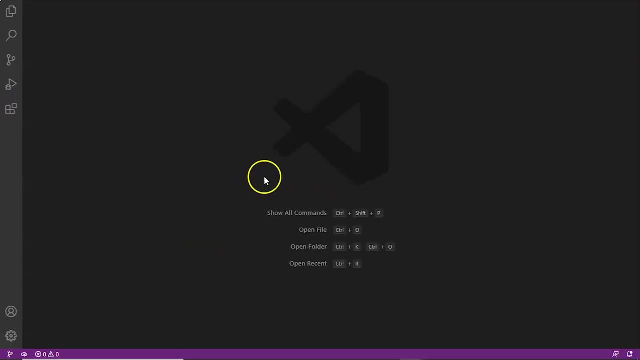 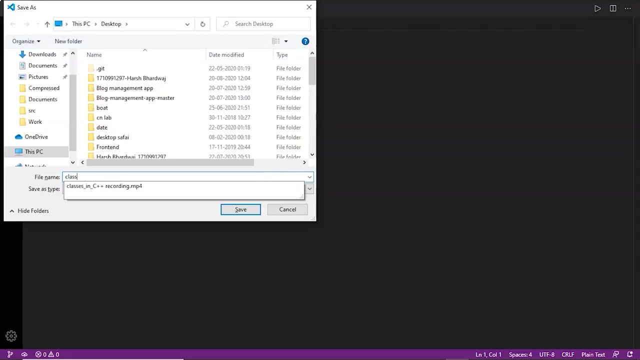 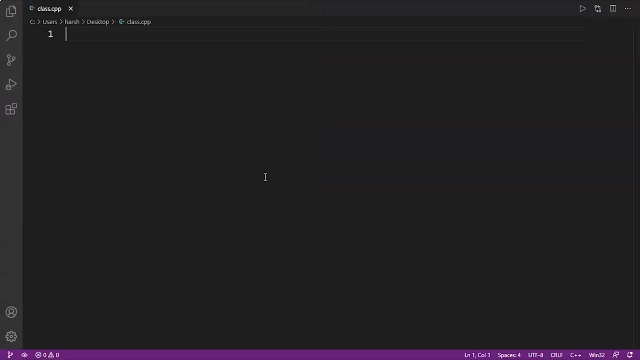 our code editor, that is vs code. now, here we will make a new file, and let's name this file as classcpp. now, here we will do a program in which we will make a class and inside that class we will make some functions, and with the help of objects of that class, we will call those functions. 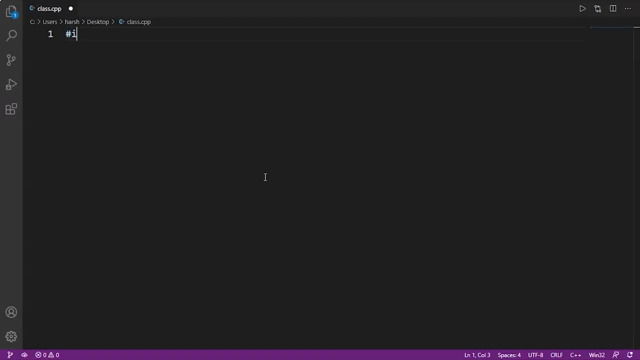 so let's start. first of all, we'll mention the header files. hash include iostream, now using namespace standard. now let's make a class and with a class keyword, and name this class as, let's say, franchise. now here, don't forget to mention the semicolon. 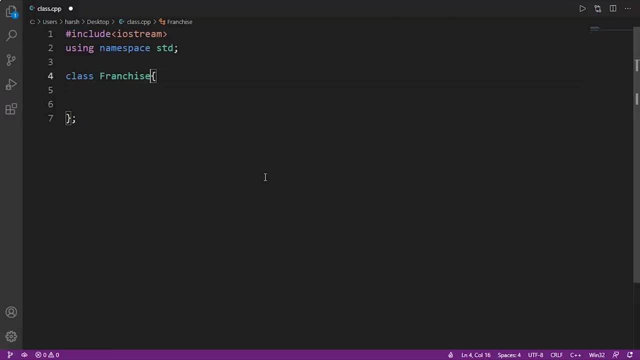 now we will write the xs modifier that is public. now we'll mention those functions. let's say void. let's name this function as kfc. now, inside this function, we will print something like: let's say: we have the best chicken. after this we'll write ndl. 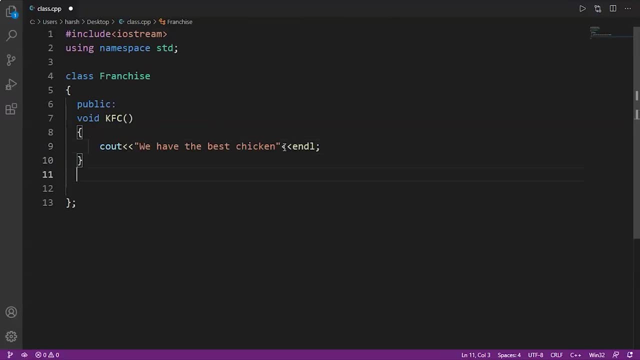 now we'll make another function named burger king, as we know that these two are famous franchise, so that is why we have put this under class for franchise. now let's print: here we have the best burgers, classic burger king. now we'll try to print these two functions with the help of object that are made from the class. 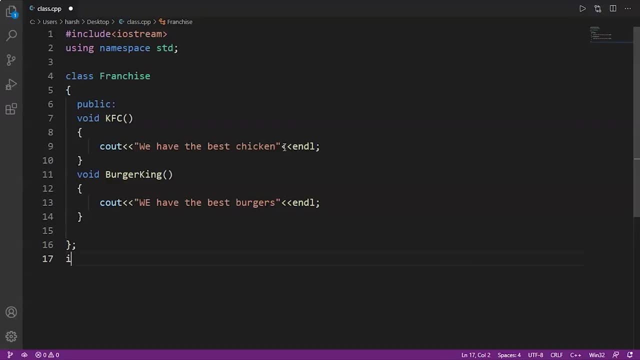 franchise. so what we'll do is we'll write and main. so what we'll do is we'll write and main. after the franchise class, we will write int main and inside this class we will make an object of class franchise. franchise is the class name, fran is the object name. now all. 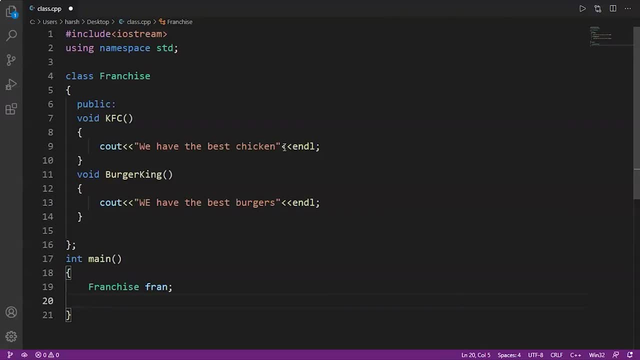 we have to do is the calling. we will call the function kfc and we will call the function burger king with the help of fran object. so let's do this: fran dot, operator kfc. that is the function name. after that we will write fran dot burger king, return zero. 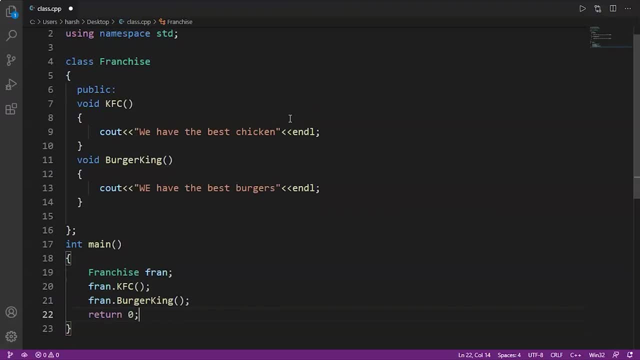 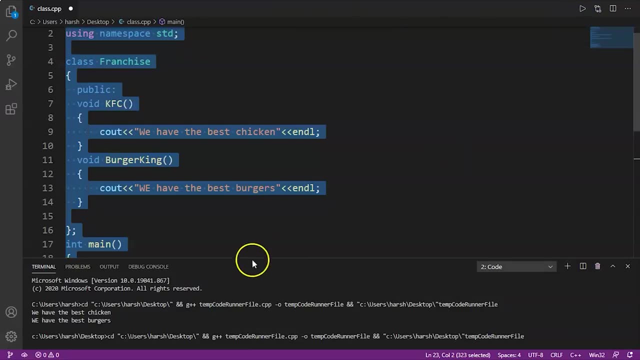 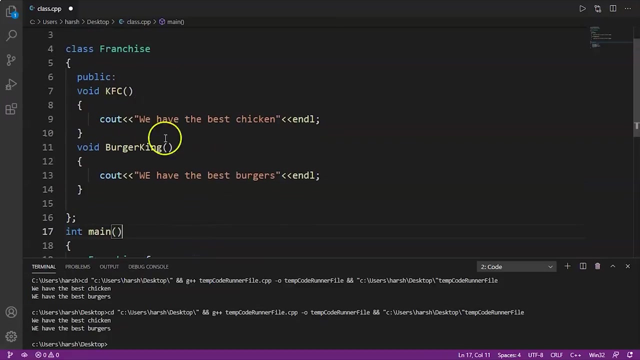 now let's try to run this one here it is actually i have run it twice, so that is why it is getting printed twice. we have the best chicken. we have the best burgers. that is what we want to print first here. fran dot kfc. call this void kfc inside this class franchise. after that, fran dot burger. 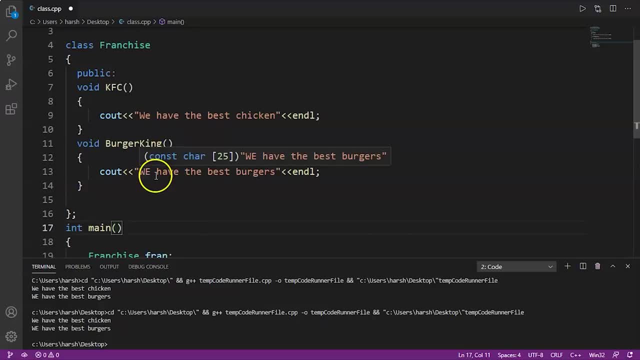 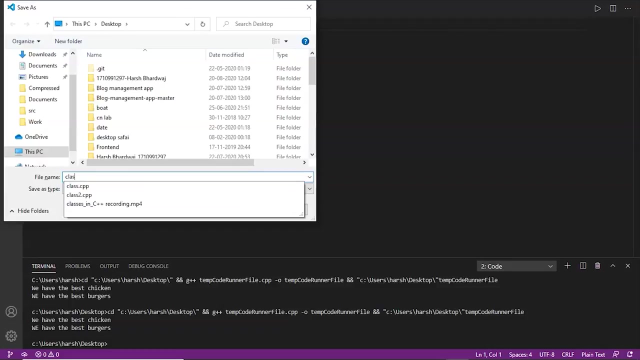 kfc king call this function burger king. so that is why they have printed serial wise: we have the best chicken, we have the best burgers. after this we'll do another example, so let's do this. first of all, we'll name this file class, class two, dot cpp. 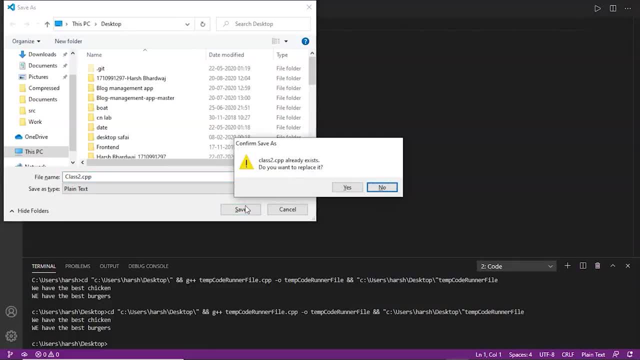 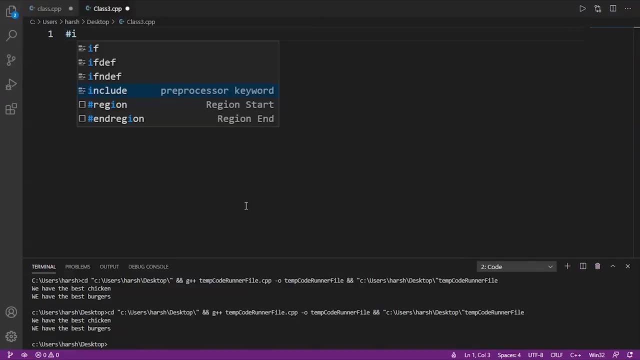 okay, i think it already exists. we have to name it something else. three: okay, now we will write the header files. hash include iostream. now, using namespace number. in this example, we will try to access a private variable, as we know that it can only be accessed from within the class. 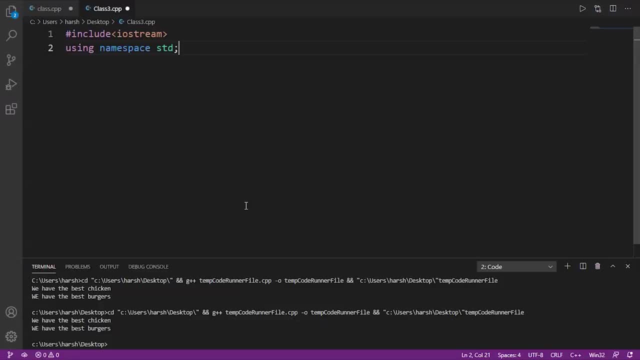 but it can be done with the help of setter getter methods. so let's start. first of all we'll write int main. now we'll make an object. for that we have to write the class name, which is billboard. we'll make this class afterwards. first of all we'll write the class name, after that we'll write object. let's name the object. 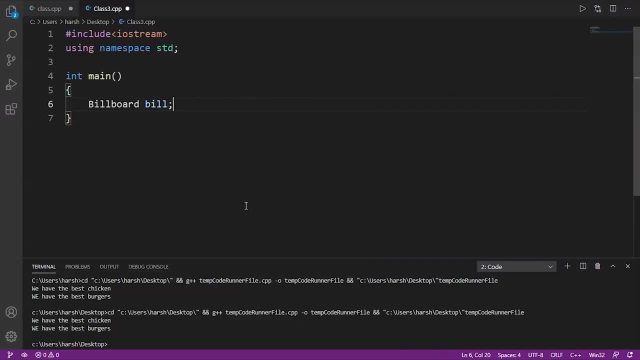 bill. billboard is class name, bill is the object name. now we will call a particular method or a function which we call setter method. we'll write bill dot. we'll name that setter method as set title. basically, this function will access or assign the value to the private. 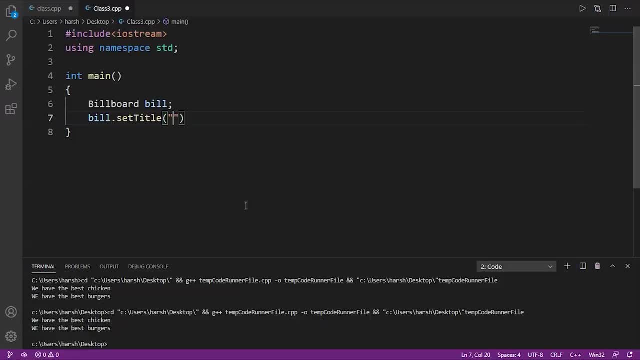 variable which we were talking about. so we'll write here, let's say, top five songs of 2020. we want this title to be written on the billboard. now we'll write the getter method, basically the setter method or set title method, will set or assign the. 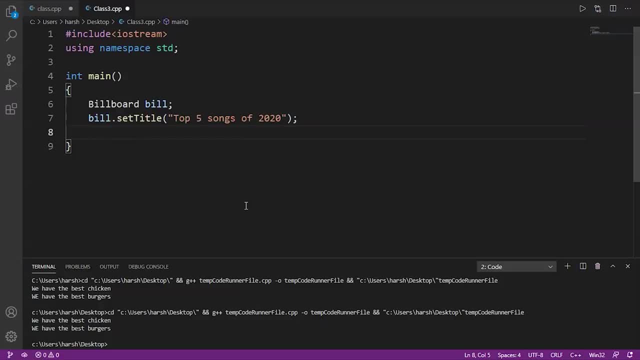 value of to the private variable and get method or get title. method will return that value from there. so we'll write bill dot. get title now because we want to print it. so that is why we'll write it in cout: okay now. after that we'll write: return zero. 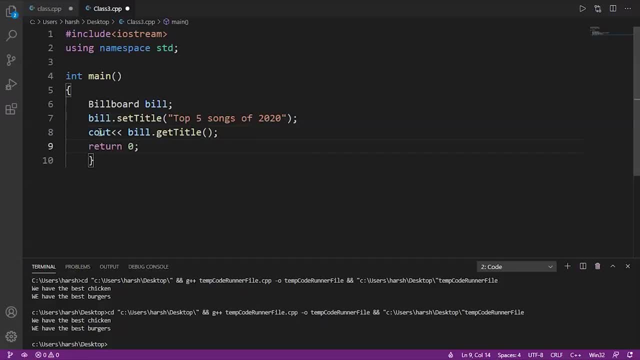 okay, now we will make the class billboard class keyword billboard. after that bracket starts. now we will write private because we want the variable to private. okay, so the data type string and the variable is title. now this variable is private and we want to assign the value to this variable, which is not possible because they are not. 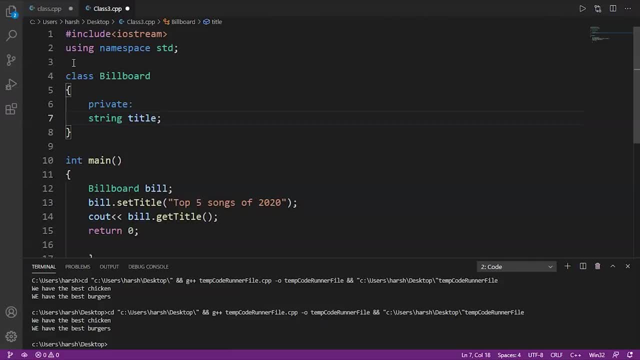 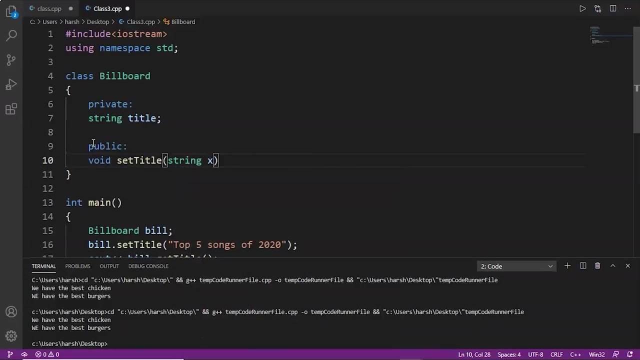 of the same class, but we will do that with the help of setter getter method. so let's do that now. we will write public- public because we want our functions to be public. now void, that is the data type, set title, and inside the bracket will write the variable. now, this method is taking this, very this parameter. 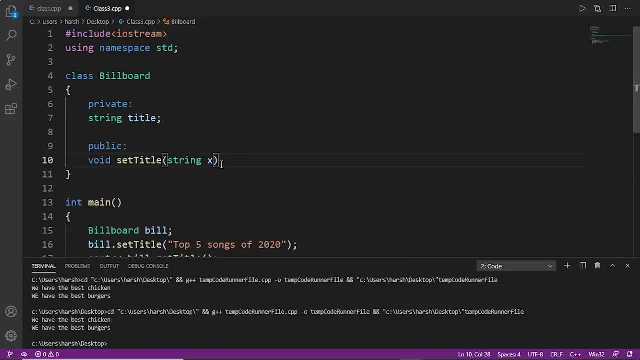 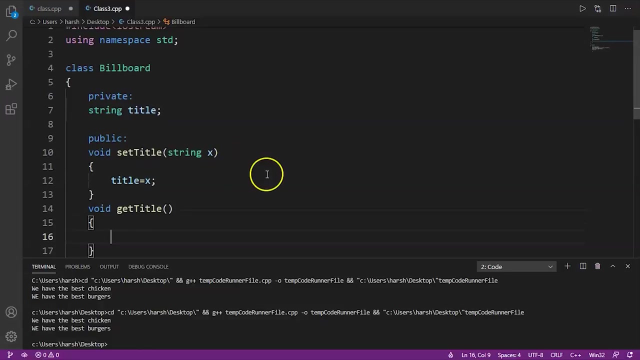 X. so we will assign this parameter X to the private variable. let's do that title. that is the private variable X. now we will write another method named getTitle. now we will write another method named getTitle now. there are no parentheses in getTitle method because this method is only returning the 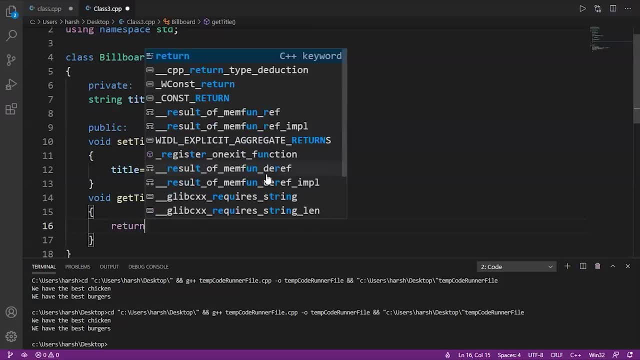 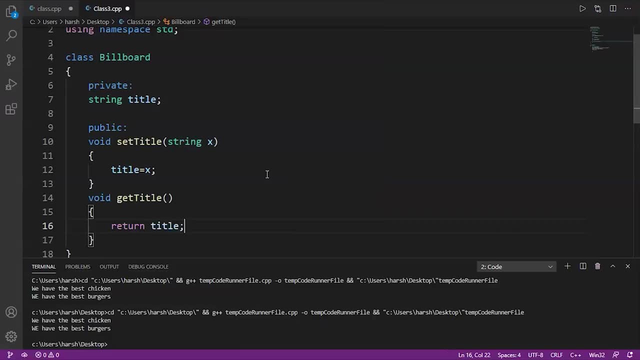 value. so we will write return title. now, getTitle function or method is returning the value of private variable title. so here what happens is that the private variable title is returning the value. so what happens is that the private variable title is returning. yeah, a minute, here is any. I will bring this digital pointer function here, so we will call it chili and 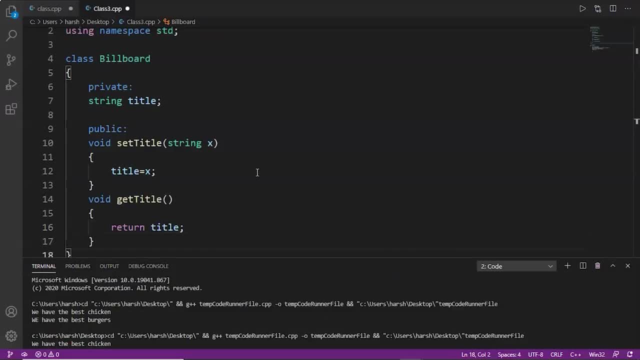 what is happening is here: the function said title, which is public, is taking a parameter X and is assigning to the title variable. so the message will get assigned to the title variable. now galera trite function is returning the value of private variable title, which is getting called in the mean function. one more thing: we forgot to put semicolon over here. 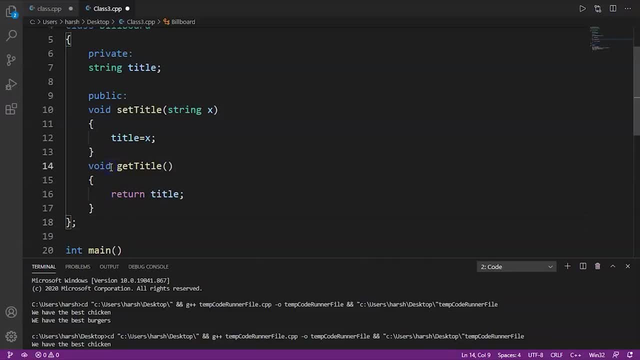 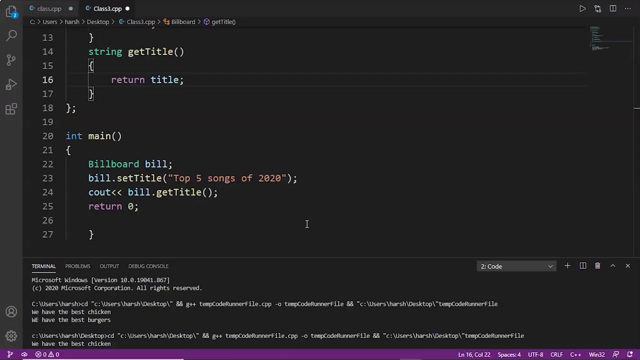 and we have written title function. we have written title function. so then it will ask for this value. this will come to the We get title cannot be void because it is returning. it would be string because it is returning some value now. So basically build dot, set title in the main function will set the value or assign the. 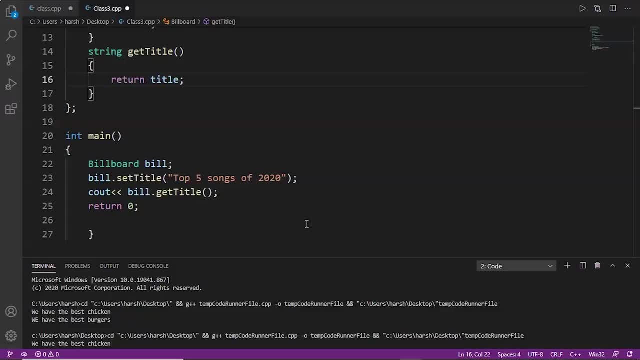 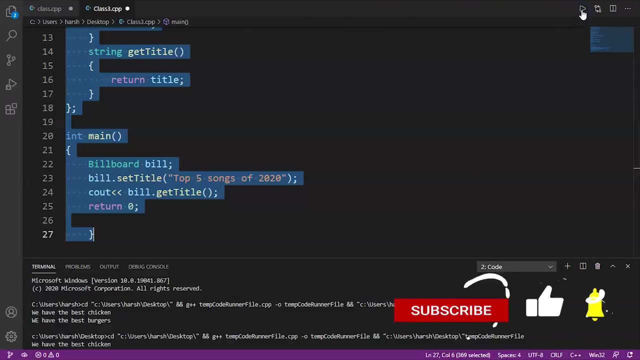 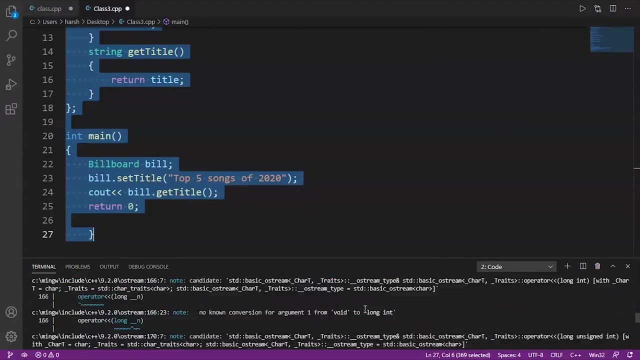 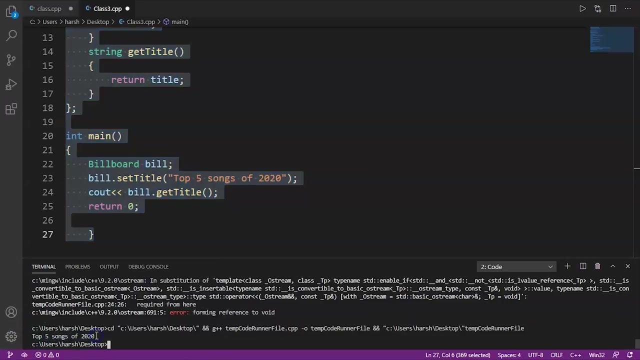 value to the private variable and build dot get title will return the value of that private variable, which will get printed. So now let's try to run this top five songs of 2020. here we can see: it is getting printed. So this is how we can do that. 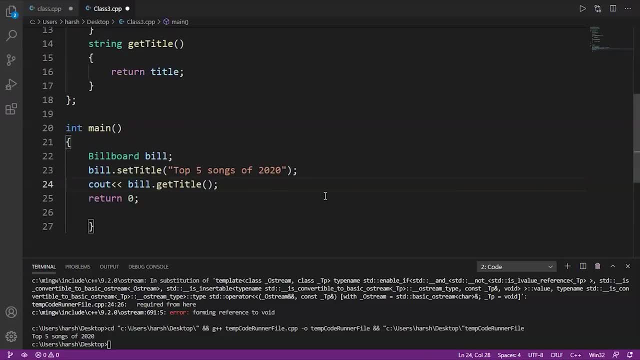 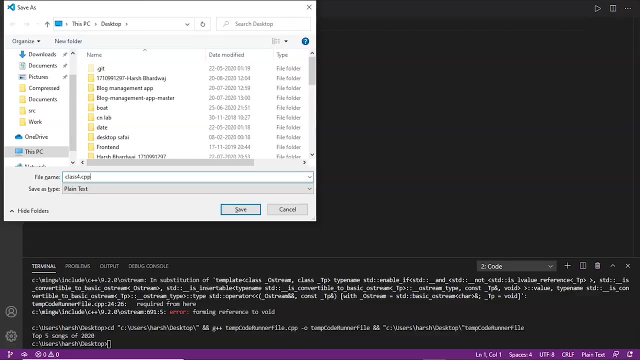 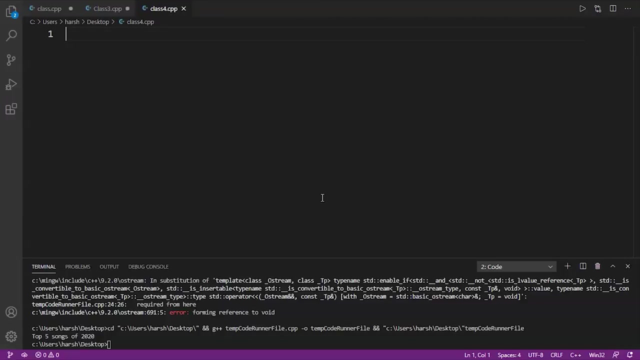 We can access the private variable using setter and getter method. Now let's do another example. Let's name this as class four, dot CPP. Now, here we will do the same example, but we will do it with the help of constructors. So let's continue. 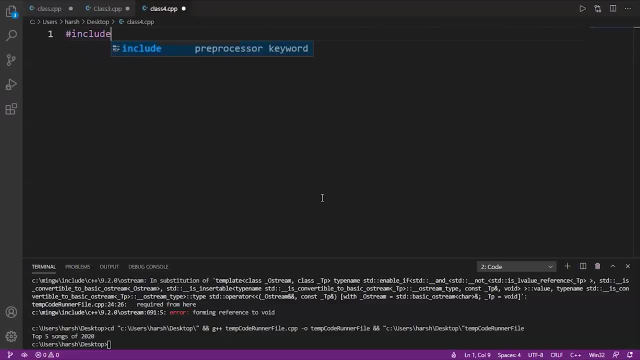 First of all, we'll write hashing. Include iostream After that, using namespace standard. Now here, first of all, we'll write int main. Now we'll name the class. We'll write the name of the class, that is billboard. 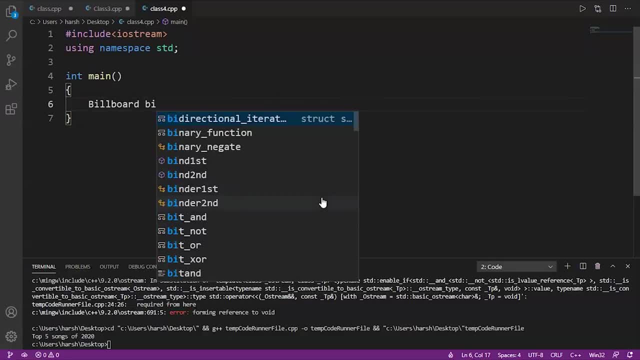 And we'll make the object of it, as we have done previously, like bill. Now we'll make a constructor of this object and we'll pass the parameters, will pass the string as top three songs of 2020.. Okay, As we are passing the string to the constructor, that means the constructor is parameterized. 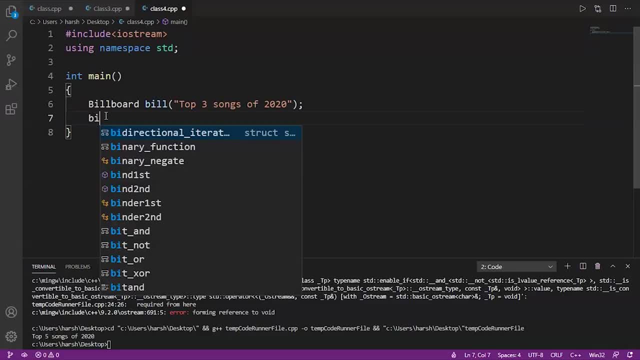 constructor. And now we'll write: bill dot get title. here we are writing this because function this function is returning the value of private variable title, So that is why we have to write it. Okay, And we'll print it. actually, cout Return zero. 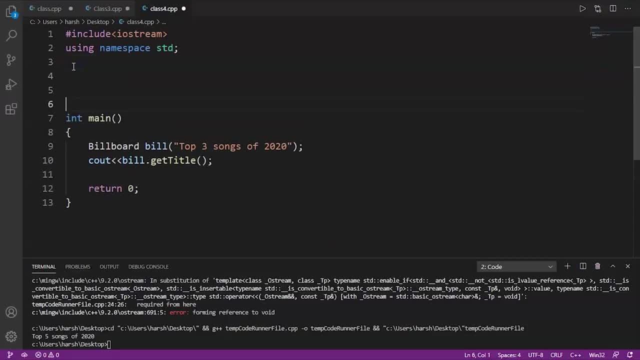 Now let's do the other thing, As we have done previously. we'll write class billboard- we are making this class. and inside this class We are making the variable private string title is private. Now we'll write public access modifier. Now, here we will write the constructor in which we were passing the string from the 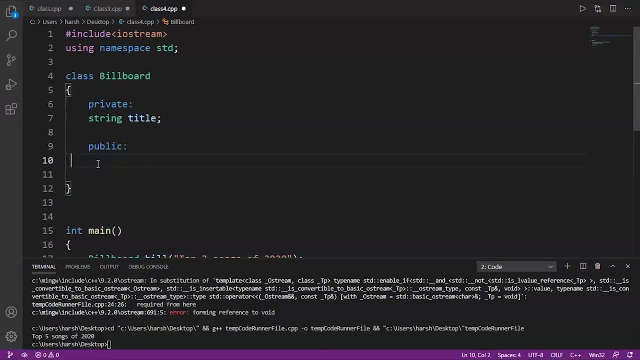 main function, So we'll write the name of the constructor. As you all know, the name of the constructor is same as that of the class, So it would be billboard And the parameter is B. that parameters which we are passing from. the main function is getting. 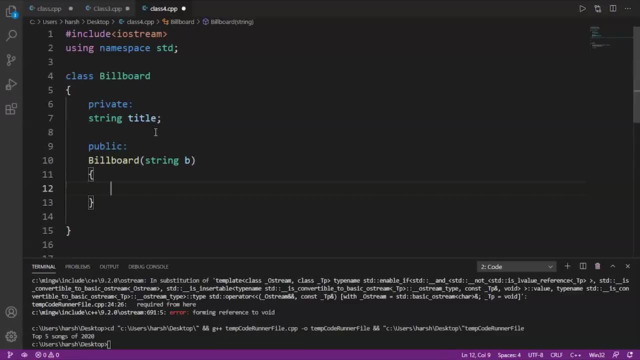 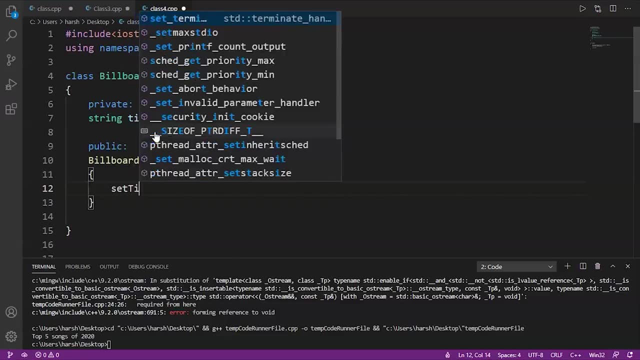 stored in B. Now, inside this constructor, we'll call the method set title. Okay, So we'll write set title. We are passing the same string to the set title method. Now we'll make this method set title. We'll write void set title. 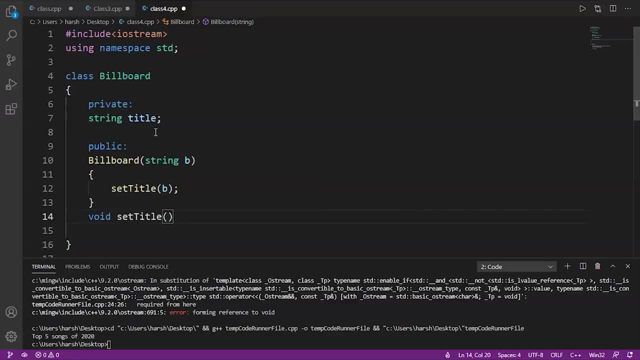 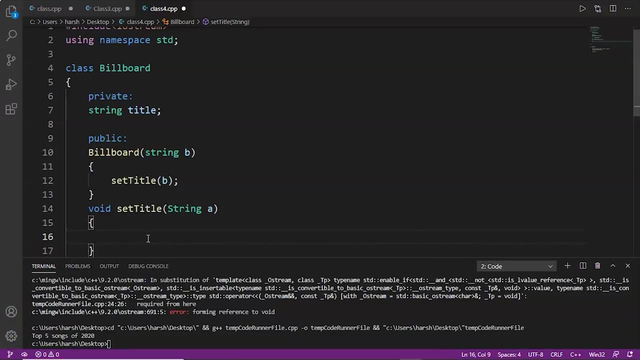 Okay, So we'll write void set title. Okay, So we'll write set title. We'll write void set title. Okay, So we'll write string A. So, actually, what is happening? we have passed a string named top three songs of 2020 to 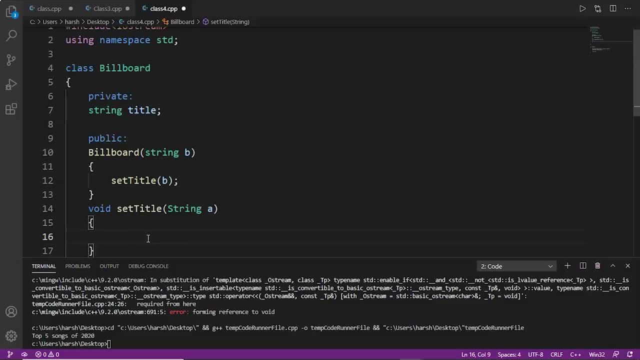 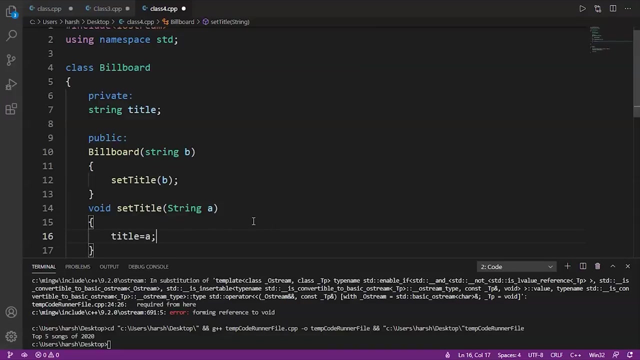 the constructor. The constructor is further calling to the method or function named set title and is passing that string to the same function. Now that function is set title And now we will assign that string to the private variable title. So let's write: title equals A. A is that string? 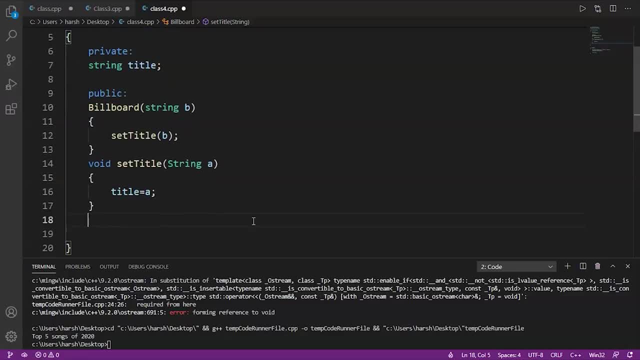 Now, as you have done previously, we'll write void: get title. Now get title function is used for returning the value of private variable, as we know, So we'll write string. actually Okay, So we'll write string: get title. string get title: return title semicolon. 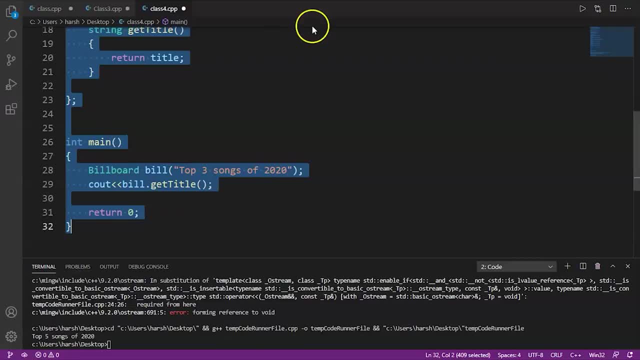 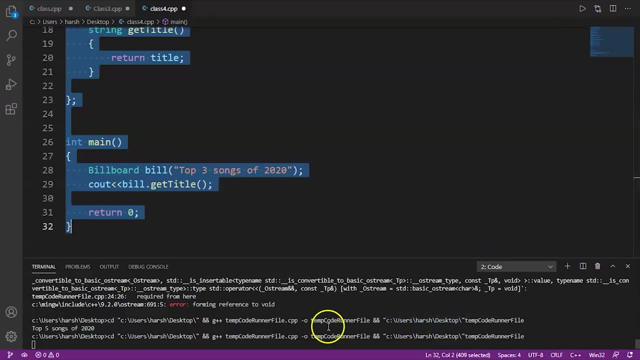 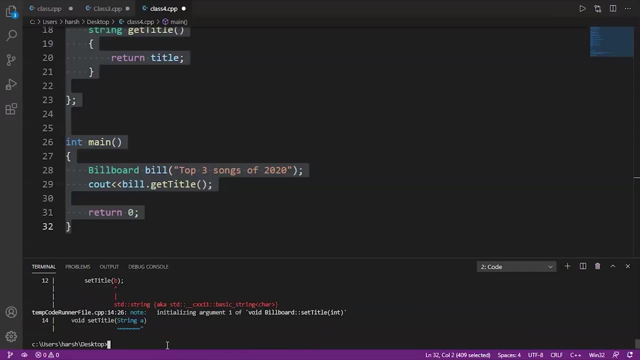 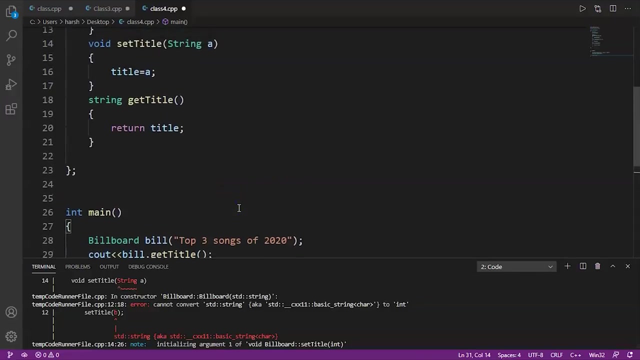 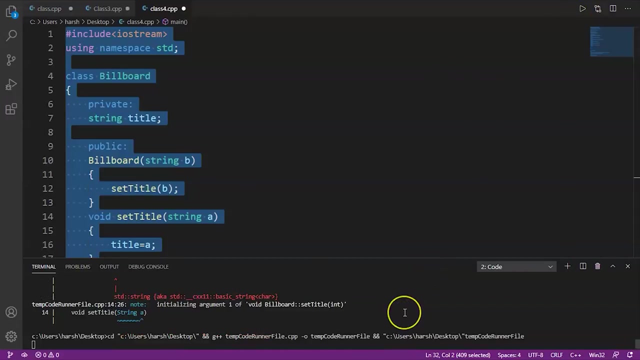 Now let's try to run it. I think something is wrong Here: capital S. we have written Here: capital S. we have written: Let's make it correct. Let's make it correct S. Now let's try to run again. we can see top three songs of 2020.. 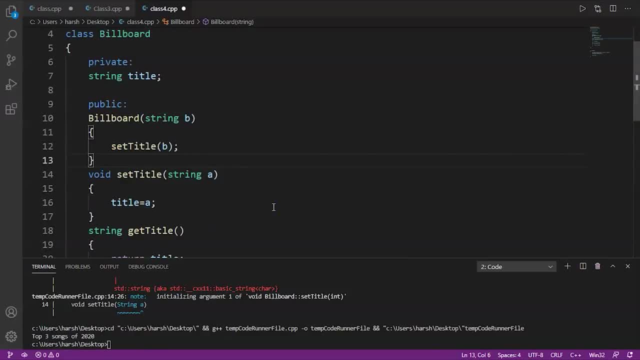 So this is how we can print with the help of constructor. This was the same example as that of the previous one, But to understand constructors, we have done this with the help of constructors and we get the right output. So after this we'll do the example of destructors. 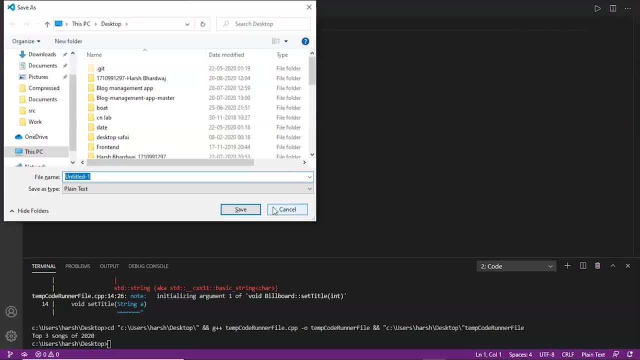 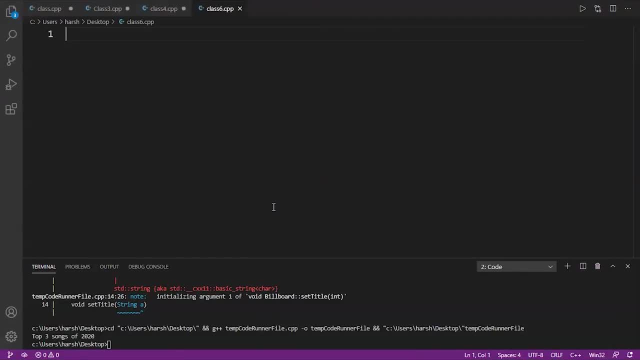 Okay, let's name this as class6.cpp. Now let's write the header files hash include iostream bring namespace standard. Now we'll start with int main. So first of all we will write the class name, that is gambit. 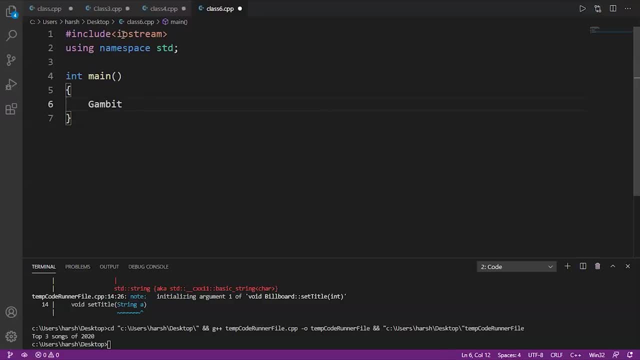 To access the class we need to have an instance or object of class. Here the name of the object is gam. After this we will call a function display. So we will write: gamdisplay returns zero. Now let me tell you what is happening. 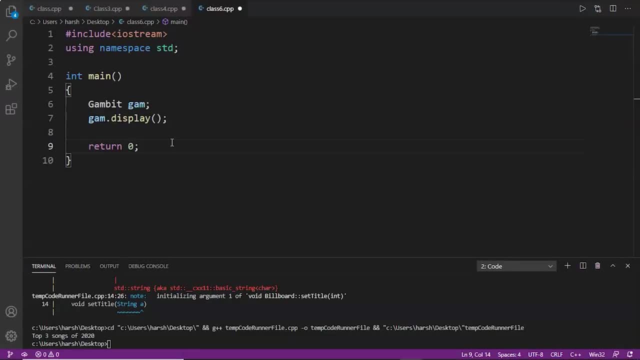 So, as we declared, this object, constructor will be called, that is, gambit and the message inside the message, The message inside the constructor, will be printed After the constructor gets completed. we will return back to the main. Now we have gamdisplay, which is used to call display function inside the gambit class. 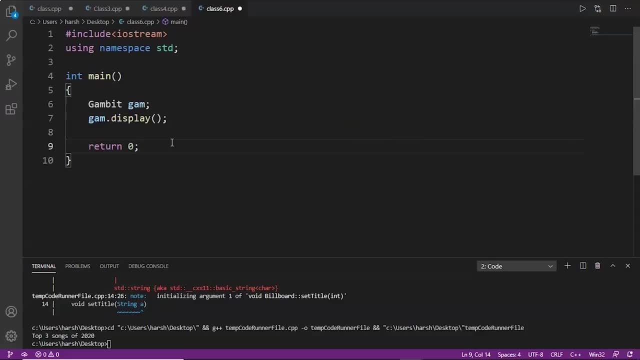 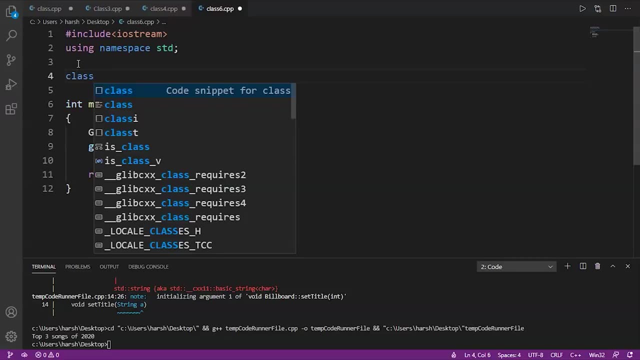 So after this we will write the class- Let's make it class keyword: gambit. Now we will write public access modifier. Now we will write the constructor, And inside the constructor we will display the message. We will write: hello, Hello. 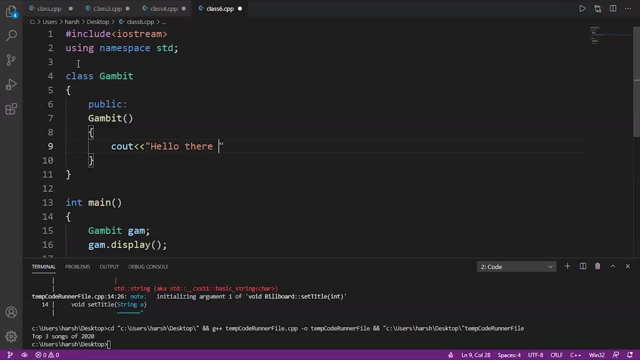 Hello, Hello, Hello there, I'm constructor. I'm in constructor. Now, here we will write the destructor: Hello Gambit. and inside the destructor we will print the message just to indicate that we are in the destructor. Hello there, I am in destructor Semicolon. But before that we have to write. 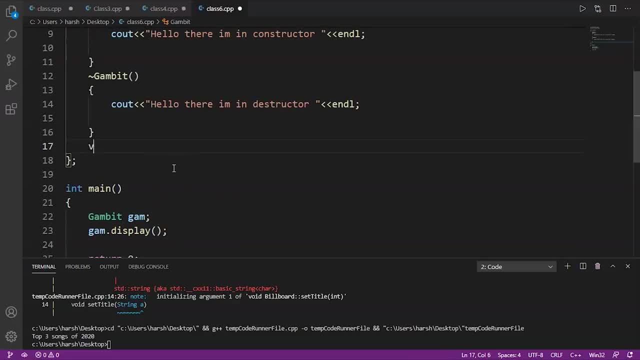 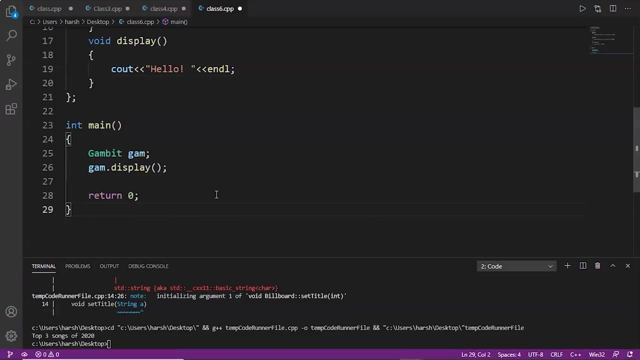 the function display also. So we will write void display and we will print the message. Let's say hello and null. Now let's try to understand this again. As the object is declared, constructor will be called- that is gambit, and the message inside the constructor will be printed After the. 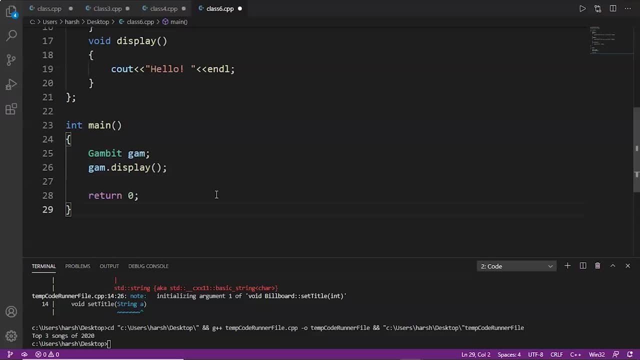 constructor gets completed, we will return back to the main. Now we have gamdisplay, which is used to call display function inside the gambit class. So hello will be printed. Now, As we can see, the program has finished the execution. Now the destructor will be called. 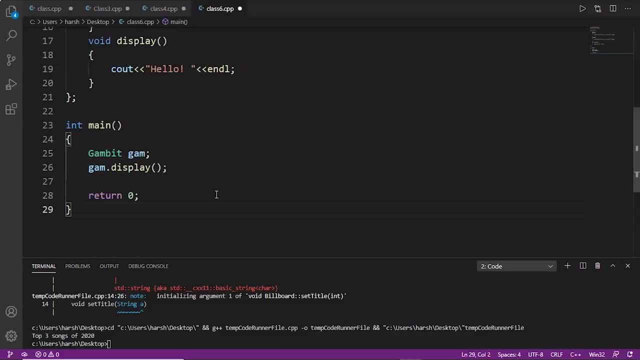 and hello I am, destructor will be printed. As we know, destructor destroy the object at as the scope of the object ends. So after the scope of the object ends, hello I am in. destructor gets printed in the last. So now let's try to run this. 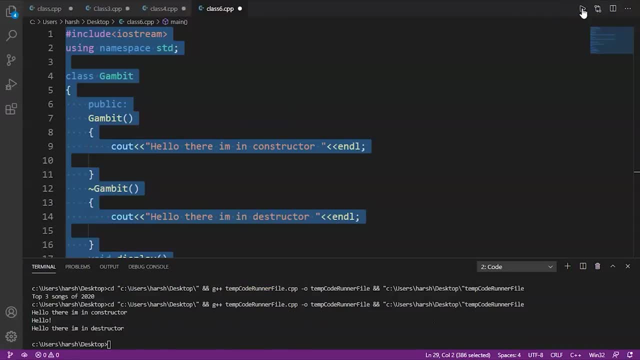 here we can see: hello, there, I'm in constructor. then hello is printed. then hello, there I'm in destructor is printed. as we have thought, destructor is getting printed in the last because, as we know that, when the scope ends, the destructor is called. so these were some. 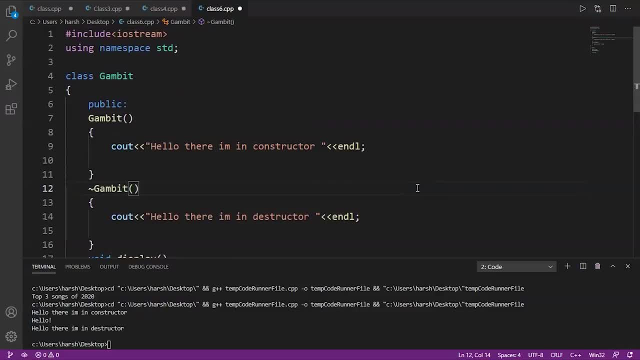 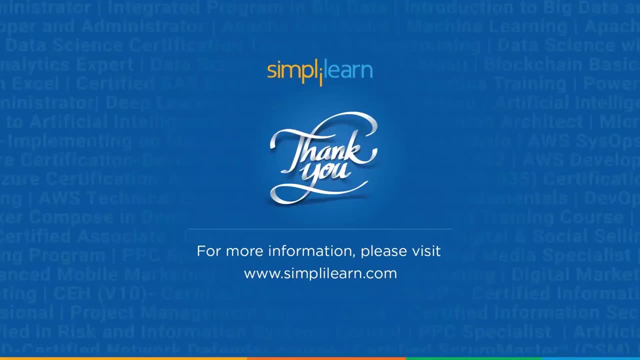 basic examples of classes in C++. in order to understand them better, you must practice some more examples on them. alright, guys, with that we have come to the end of this video. if you like this video, please give it a thumbs up. I hope it really helped you all thanks. 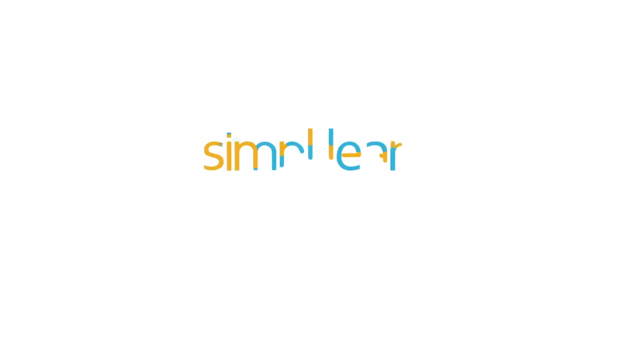 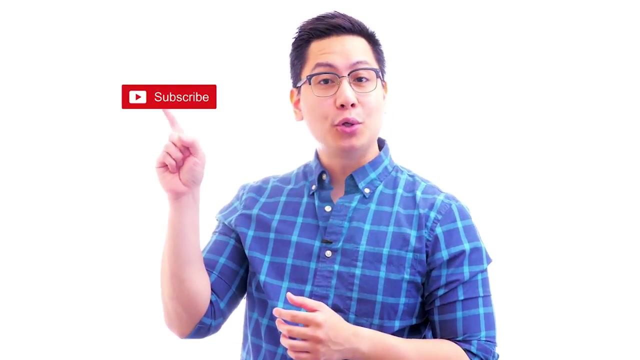 for watching, stay safe and keep learning hi there. if you like this video, subscribe to the simply learn YouTube channel and click here to watch similar videos. to nerd up and get certified: click here.